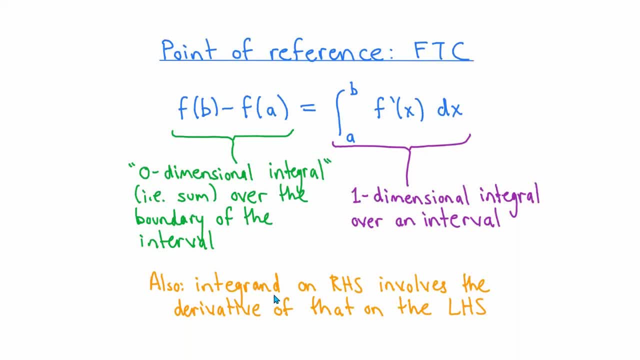 These three features of the Fundamental Theorem of Calculus form a pattern that you can see repeated in Green's Theorem and Stokes' Theorem and in the Divergence Theorem in the next video. One of the main differences is that in Green's and Stokes'. 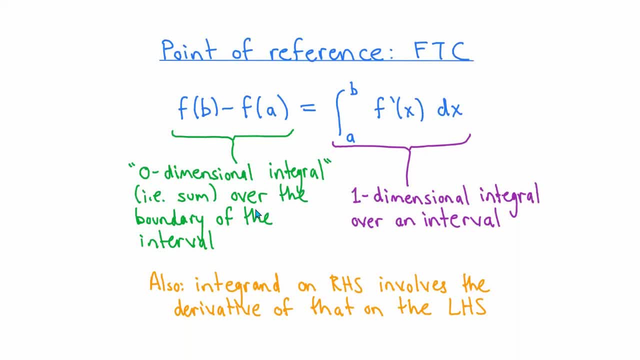 Theorem, the integrals involved are two and one-dimensional, while in the Divergence Theorem they're three and two-dimensional. There are also some other differences with what exactly the integrands look like, but we'll see those when we get to the precise statements of the theorems. 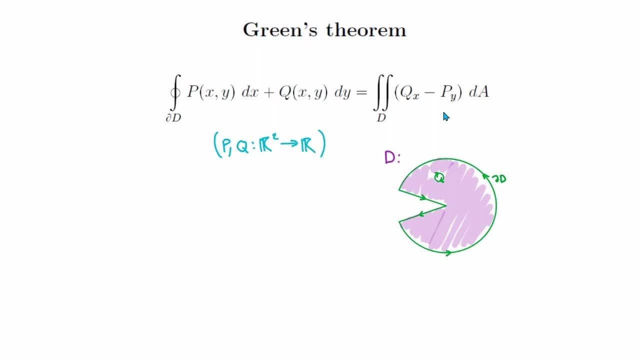 Now let's try to understand the statement of Green's Theorem. Green's Theorem says that for a region d in the plane and functions p and q from r2 to r, the oriented integral over the boundary of d of pdx plus qdy is equal to the double integral over d of the partial of q, with. 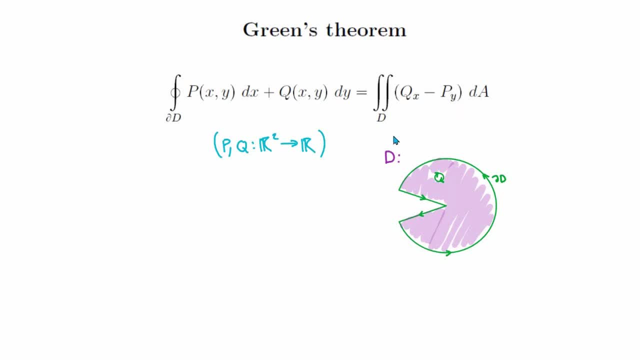 respect to x, minus the partial of p with respect to y. This may seem like a lot to digest when you first look at it, so it's helpful to see how it fits the pattern that we just described. First of all, the object on the right-hand side is a two-dimensional integral over a region d in. 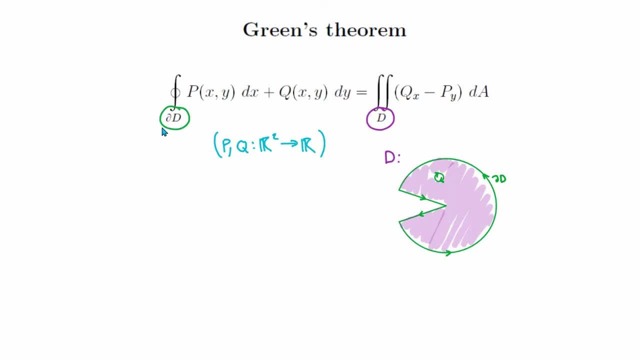 the plane. Second, the object on the left-hand side is a one-dimensional integral over the boundary of the region. The circle on the integral on the left indicates that we're taking the boundary with the positive orientation, but the 2-dimensional integral on the left-hand side indicates that we're taking the 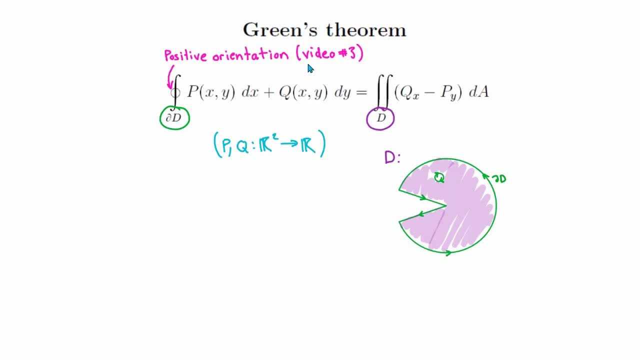 orientation. If you want to remind yourself what the positive orientation is, you can see video number 3 in this series. It's also worth mentioning that the one-dimensional integrals on the left-hand side are line integrals of the second kind, As a matter of notation. 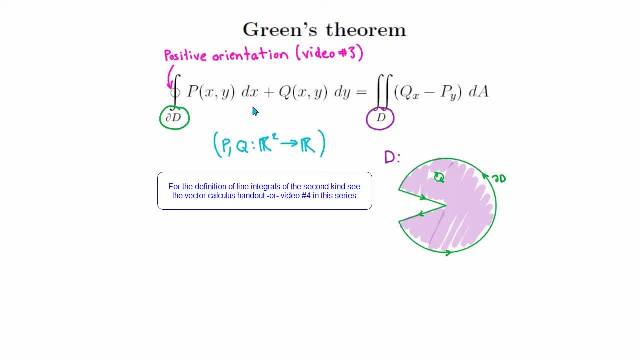 when we write the integral of pdx plus qdy, we really mean the sum of the two line integrals: integral of pdx plus integral of qdy. Most people prefer to write that this way, though, for aesthetic and typographical reasons. The third thing that you should notice about this: 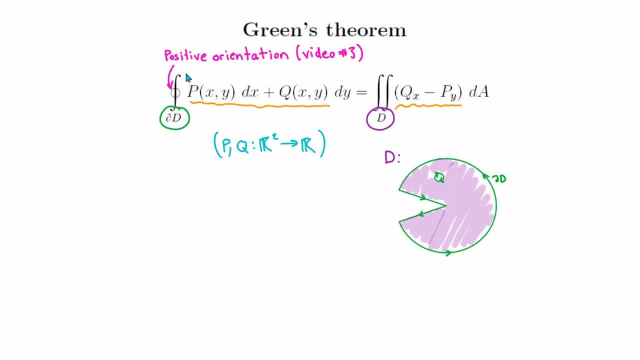 formula is that the integrand on the right-hand side involves the derivatives of the integrand on the left-hand side. Of course, there are some assumptions that need to be made in order for this formula to hold, and we're glossing over that. But in practice we are going to. 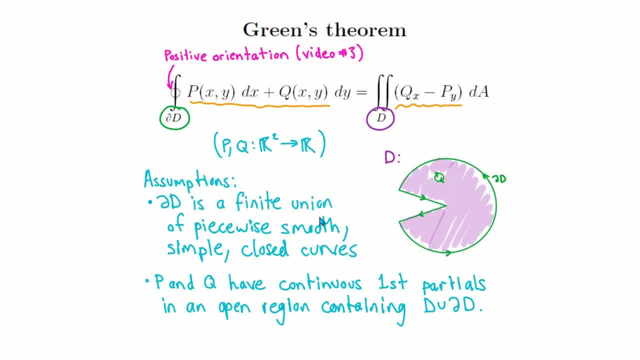 want to assume things like that the boundary is a finite union of piecewise, smooth, simple, closed curves and that p and q have continuous first partial derivatives. in an open region which contains d and its boundary, There are a lot of different applications of Green's. 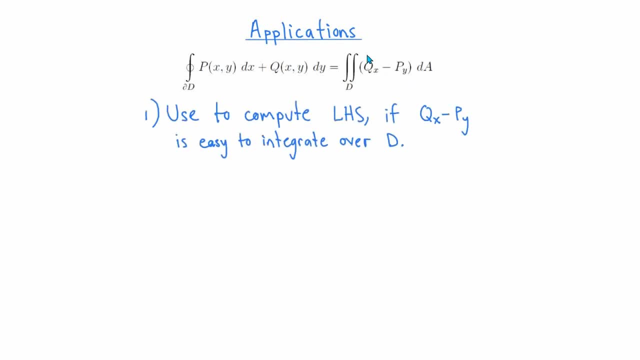 theorem, and just to mention a couple. if it turns out that the integrand on the right-hand side is related to the integral of pdx plus qdy, then we're going to want to assume that it's relatively simple. Then Green's theorem gives an easy way to compute the line integral. 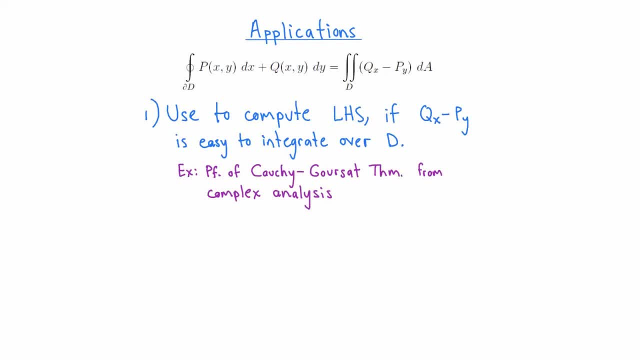 on the left-hand side. An example where you can see an application like this is in the proof of the Cauchy-Gorszot theorem from complex analysis. If you want to see the details of how this works, you can check out video number 4 of the Essential Extract Complex Analysis. 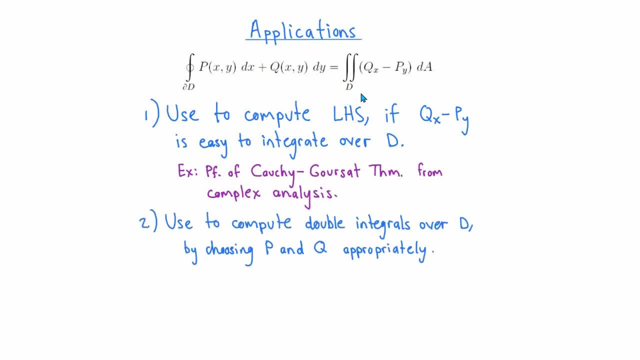 series. I'll put a link to that video above. A second way that Green's theorem is sometimes applied is to compute double integrals over certain regions d by choosing p and q appropriately and then computing the line integrals on the left-hand side. 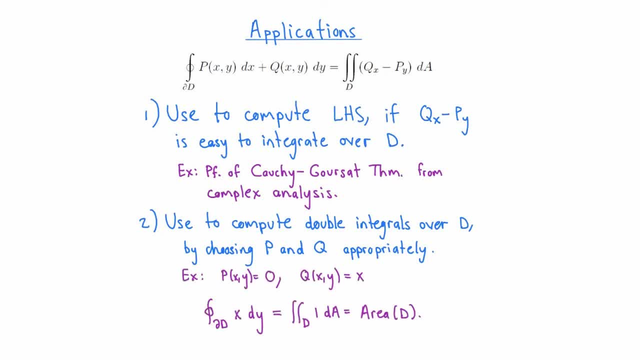 There are a number of interesting applications like this, but just to give you the flavor of what I mean, let's suppose that you just want to compute the area of some region in the plane. Well then, you can make any choice of p and q with the property that qx minus. 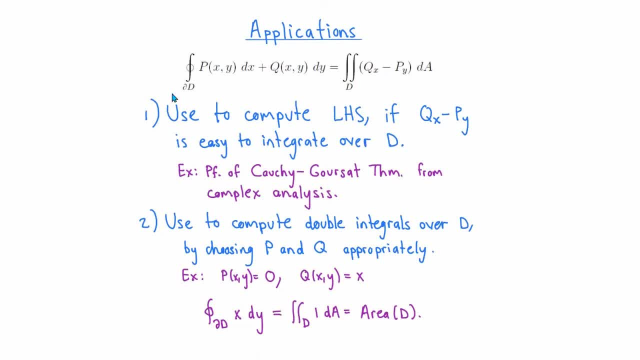 py is equal to 1.. As long as you can compute the line integrals on the left-hand side, what you get is going to be equal to the area of the region that you're interested in. One possibility is to take p equal to 0 and q equal to x, but there are other possibilities. 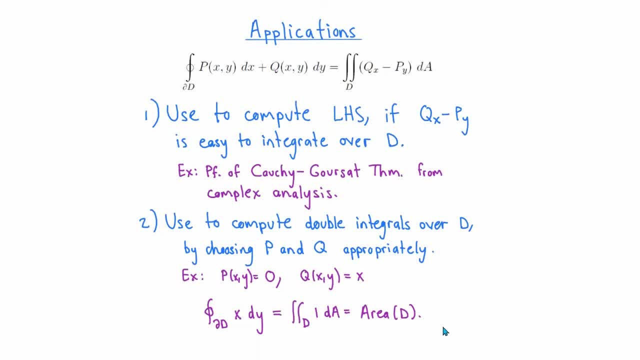 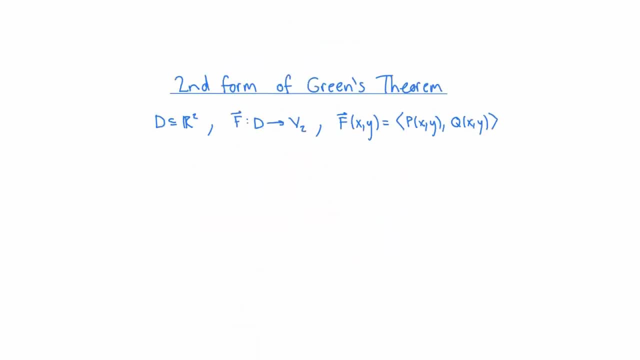 as well. This leads to some interesting mathematical formulas and it also leads to some interesting applications for engineering. Before moving on to the statement of Stokes' Theorem, let's talk about a second and third form of Green's theorem which you might encounter. The second form of Green's theorem is what? 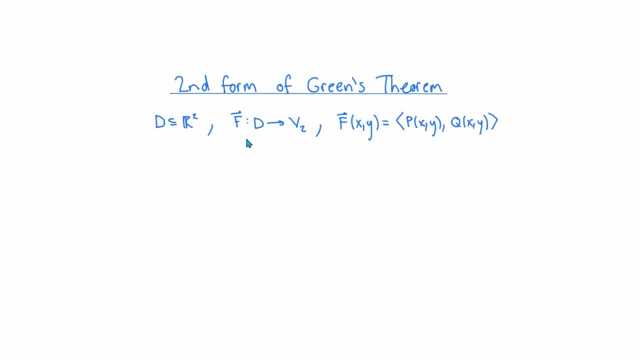 I would call a vector form of Green's theorem Here. let's suppose that we have a vector field, f, defined on some region d in R2, and let's suppose that the component functions of our vector field are p and q. Consider the line integral of the third kind, integral. 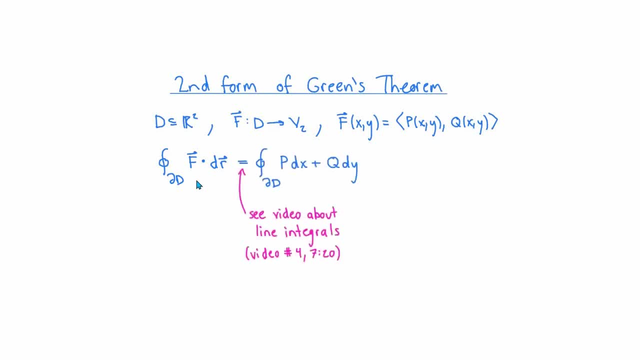 around the boundary of d of fdr. You might remember that this line integral is equal around the boundary of d of pdx plus qdy. If you didn't know this, or if you can't remember why this is true, you can see the derivation in video number 4.. Just, 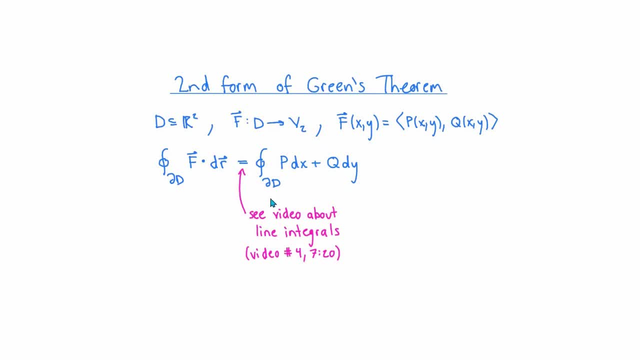 fast forward to the 720 mark in that video. Combining this observation with the statement of Green's theorem immediately gives the formula that the integral around the boundary of d of f, dot, dr is equal to the double integral over d of qx minus py. This is an important form of Green's theorem and, as 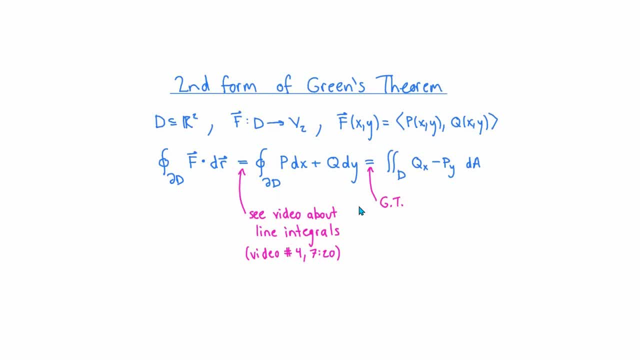 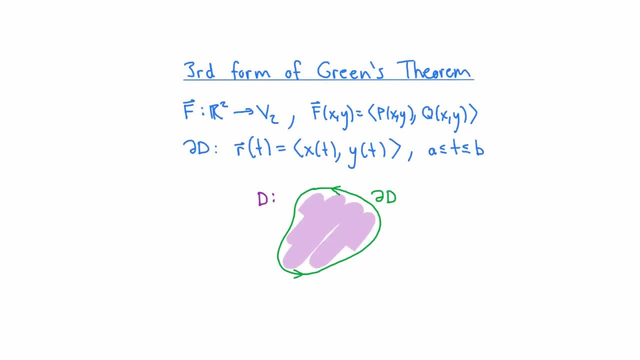 you'll see later in this video. it paves the way for the generalization to Stokes' theorem. The third form of Green's theorem is what I would call a divergence form of Green's theorem and it takes a little bit of setup to state. 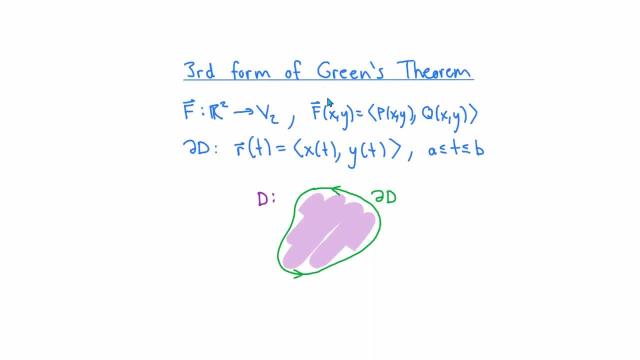 it Just as in the second form of Green's theorem. let's suppose that f is a vector field from R2 or from some sub-region d of R2 to V2.. The component functions of f again are p and q, and this time let's parametrize the boundary of d with the 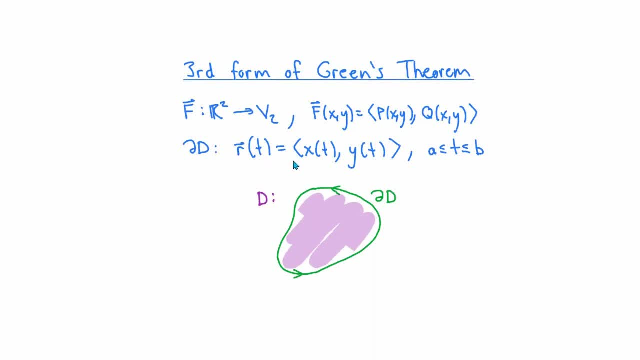 positive orientation by a vector function, R of t, whose component functions are x of t and y of t, with t running from a to b, In order to state the third form of Green's theorem, I want to define a U of t and I want to define a U of t, and I want to define a U of t and I want to. 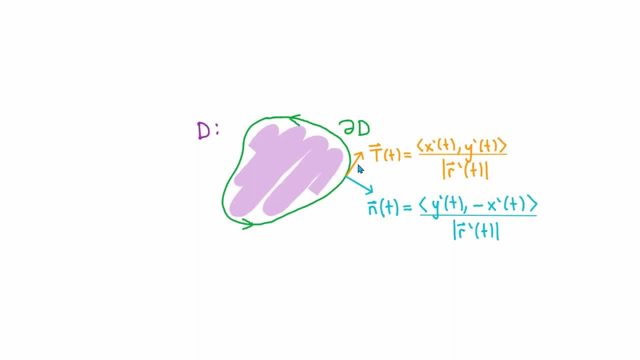 define a unit normal to the curve boundary of d. Remember that the vector function T of t, defined by x prime, y prime divided by length of R prime, gives a unit tangent to this curve at every point. It's not difficult to see that the 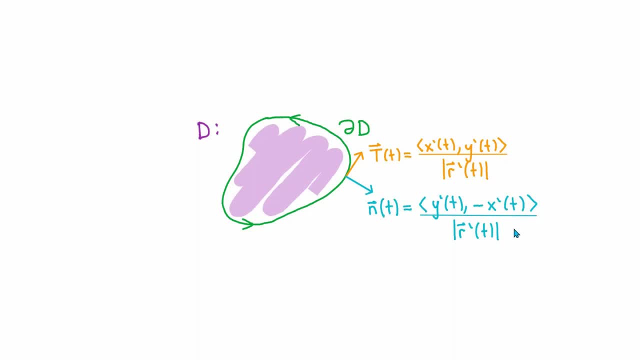 vector function, y prime comma minus x prime divided by length of R prime is perpendicular to the unit tangent and also has length 1.. Therefore this defines a unit normal vector to the curve at every point. Now let's consider what we get when we integrate f, dot n ds around the 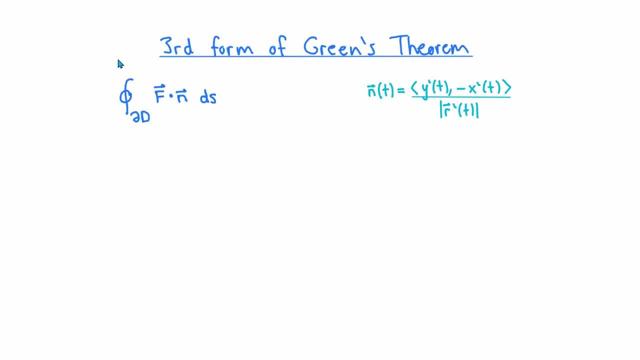 oriented boundary of d. Notice that this is a line integral of the first kind, Using our parametrization and the definition of line integrals of the first kind. this is the integral from a to b of the quantity that you see here When we multiply the length of R prime of t through. this simplifies and you might. 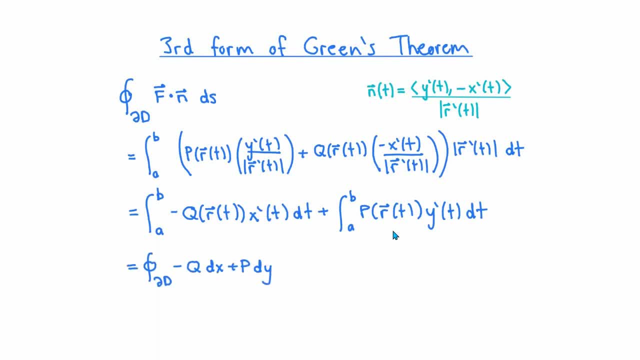 recognize that it's now a sum of two line integrals of the second kind. Now, applying Green's theorem to this quantity, with minus q playing the role of p in the original statement of the theorem and p playing the role of q in the original statement of the theorem, 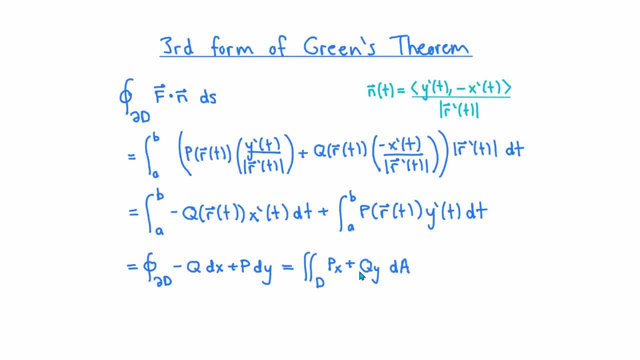 we find that it's equal to the double integral over d of px plus qy. You might recognize that this is precisely the divergence of the vector field. That's the reason why I called this the divergence form of Green's theorem. It says that the integral over the oriented 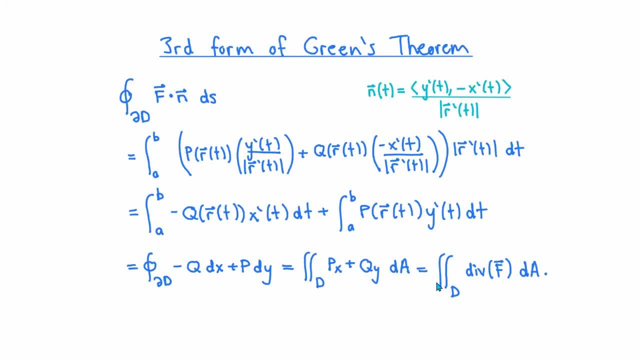 boundary of d of f, dot, n, ds is equal to the double integral over d of the divergence of the vector field. This form of Green's theorem paves the way for our generalization to the divergence theorem in the next video. Now let's move on and talk about Stokes' theorem. Before we present the statement of Stokes'. 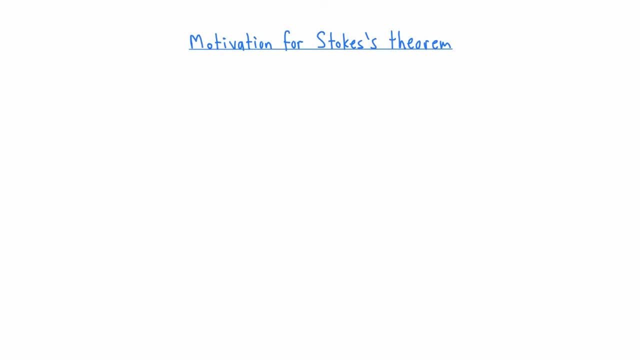 theorem. I'd like to take a minute to talk about the motivation for this theorem and to try to explain how it relates to Green's theorem. Green's theorem gives us a relationship between the double integral over a region d in the plane and line integrals over the. 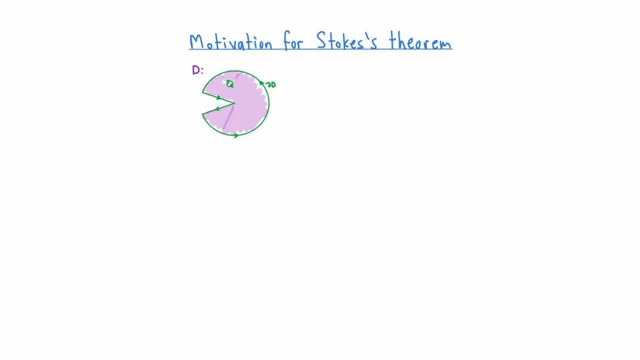 boundary of the region. However, since a lot of physics is three-dimensional, for applications to physics we'd like to have a version of Green's theorem where the double integral is not over a region d that's contained in the plane, but over a surface S that's contained. 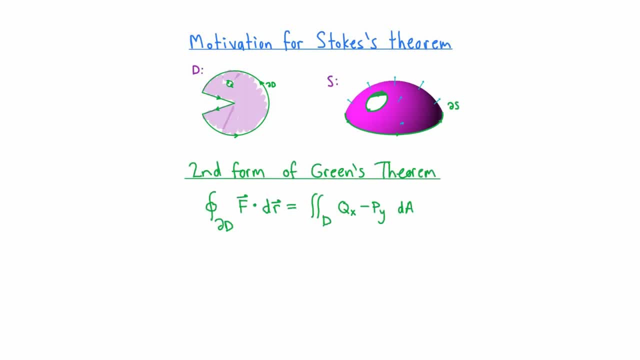 in R3.. One of the ways to see how such a generalization is possible is to look at the second form of Green's theorem. When we derived this form of Green's theorem, we were thinking about the vector field f as being a two-dimensional. 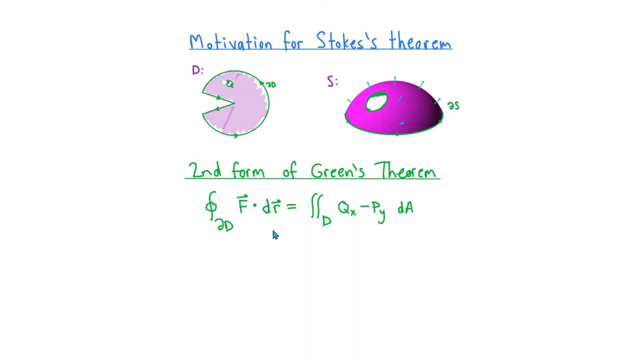 vector field. However, the left-hand side of this equation makes sense, even if f is a vector field in three dimensions. If we decide to think about f as a vector field in three dimensions, then we might also notice that the integrand on the right-hand side. 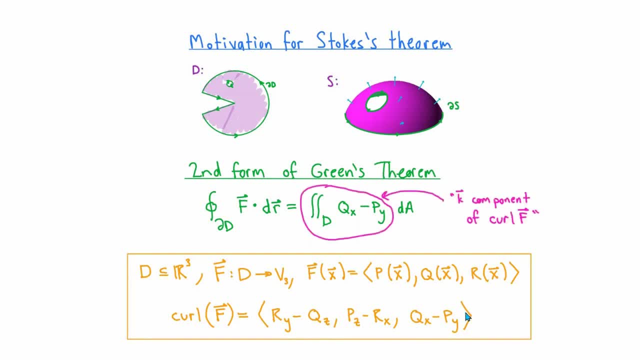 of the second form of Green's theorem is precisely the k-component of the curl of f. This observation leads directly to the generalization of Green's theorem. Now let's look at Green's theorem to surfaces, which is known as Stokes's theorem. What Stokes's 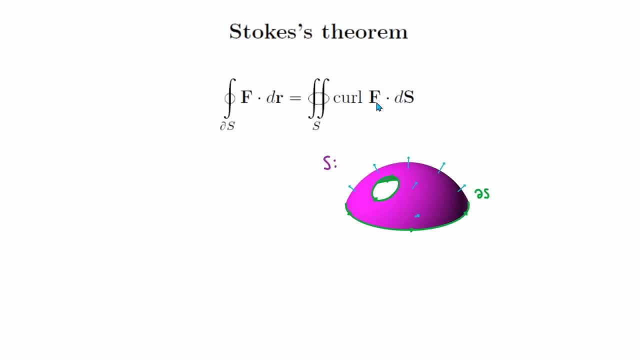 theorem says is that for a vector field f in R3 and a surface S in R3, the oriented integral of the curl of f dot ds over the surface S is equal to the oriented integral of f dot dr over the boundary of S. Once again, in order to digest this formula, it's helpful. 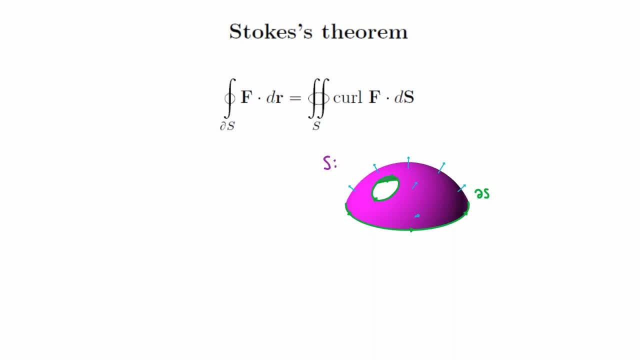 to notice that it follows the same pattern that we saw in the fundamental theorem of calculus at the beginning of this video. The integral on the right-hand side is a two-dimensional integral. It's a surface integral of the second kind over the surface S The integral on the left-hand. 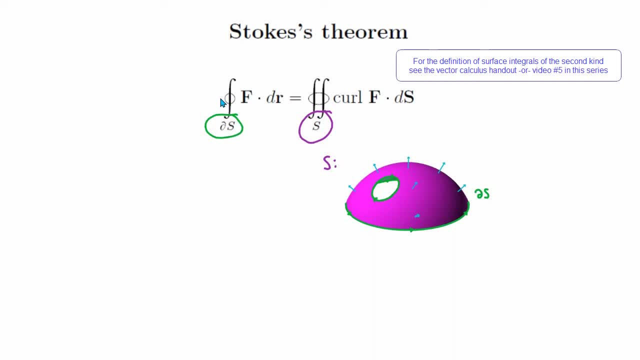 side is a one-dimensional integral. It's a line integral of the third kind over the boundary of S. Here orientation is important. We're assuming that S is an oriented surface and we're assuming that the boundary of S is given the positive orientation. with respect to the orientation, 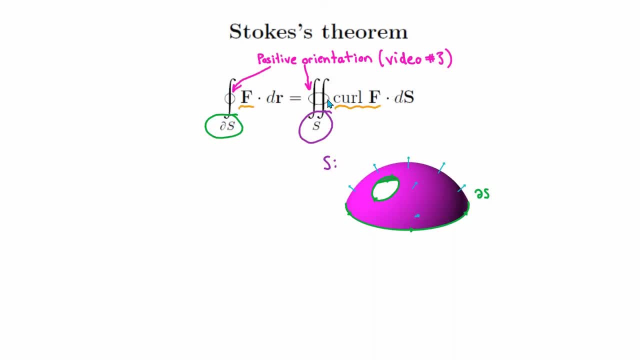 on S. Finally, notice that the integrand on the right-hand side, the curl of f, is something which involves the derivatives of the integrand on the left-hand side. Once again, there are some assumptions that we need to make, But as long as the surface S and the vector field. 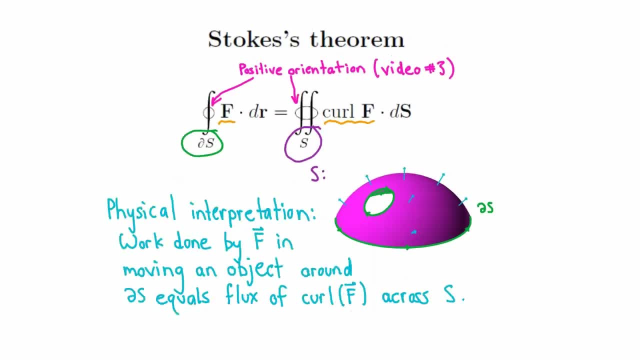 f are nice enough. the statement of Stokes's theorem is going to hold As indicated by our discussion of applications to physics. Stokes's theorem has a physical interpretation. What it tells us is that the work done by a force f- and moving an object, 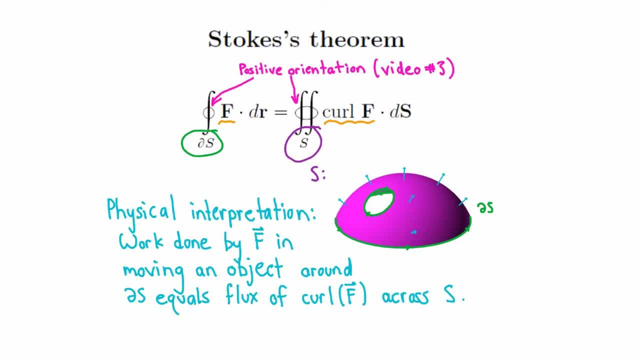 around the boundary of S is equal to the flux of the curl of f across S. If you understand the statements in this sentence and you have a good physical intuition, then you can probably figure out why this should be true. What we're saying here is that the flux on the curl of 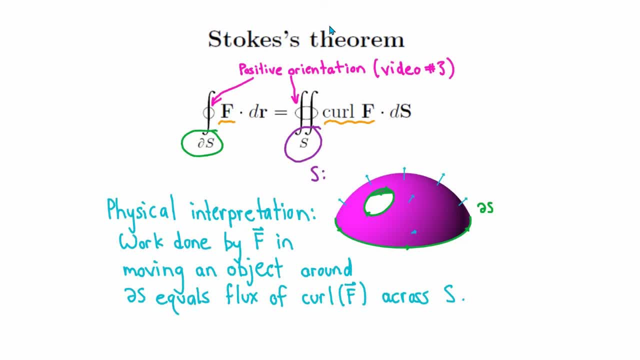 f is equal to the curl on the boundary of S. The distribution of F is also equal to the curl of F, and if you can figure out why the circle of f is equal to the curl of S you can, is that under reasonable assumptions it's actually a mathematically provable theorem. 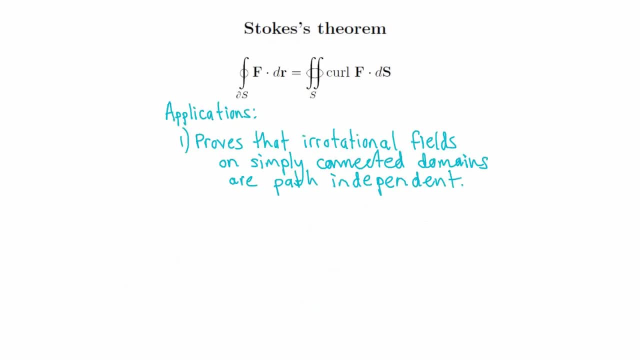 To conclude this video, I'd like to mention two nice applications of Stokes' theorem. First of all, Stokes' theorem gives us a simple proof that irrotational fields on simply connected domains are path independent. This is something that we talked about in the previous video. It's 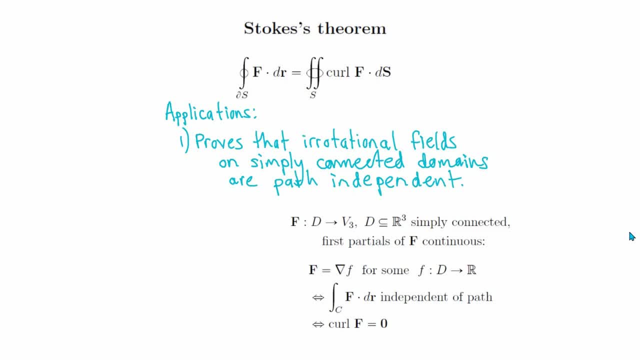 summarized near the top right hand side of the vector calculus handout in the part that looks like this: What we're trying to say here is that Stokes' theorem gives an easy proof that if the curl of a vector field, f in three dimensions is zero, then line integrals of the vector field are: 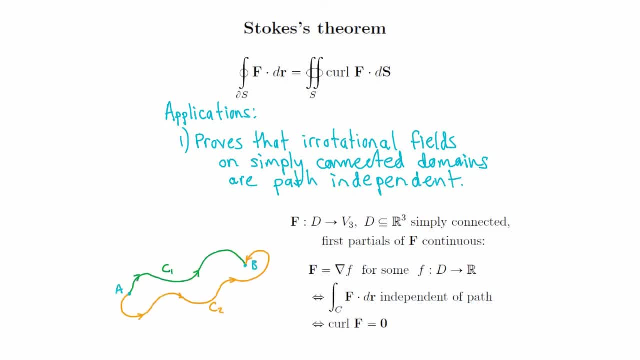 independent of path. Without trying to give a fully rigorous proof, it's relatively easy to see why this is true. Let's suppose that we have an irrotational vector field in R3, in other words a vector field that has curl zero, And let's suppose that we have two curves, C1 and C2,. 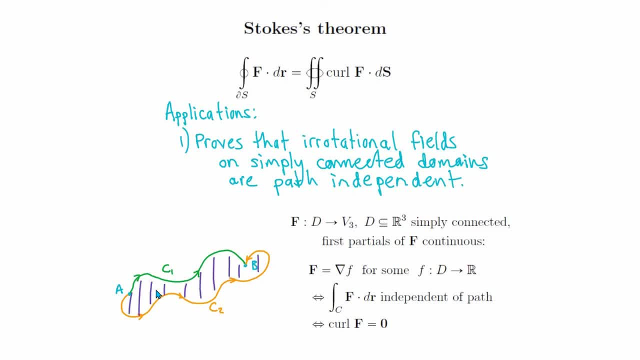 connecting points A and B in R3. Think of the curves C1 and C2 as being the boundary of a surface in R3, and think about what happens when you compute the line integral of the third kind of f of the vector field f in three dimensions. If the curl of a vector field f in three dimensions 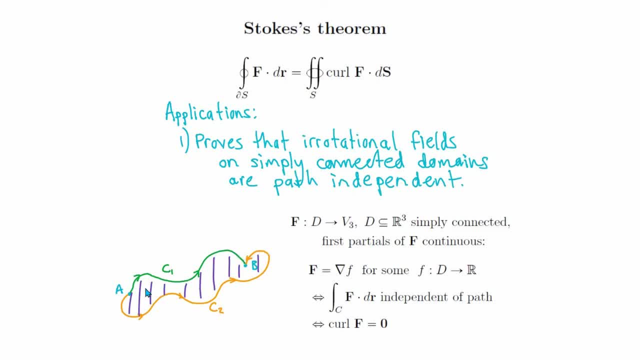 is zero, then line integral of f dot dr along C1 and then backwards along C2.. By Stokes' theorem that line integral should be the double integral over the surface of the curl of f, but by our assumption that the curl is zero, that double integral is zero. That shows that the line 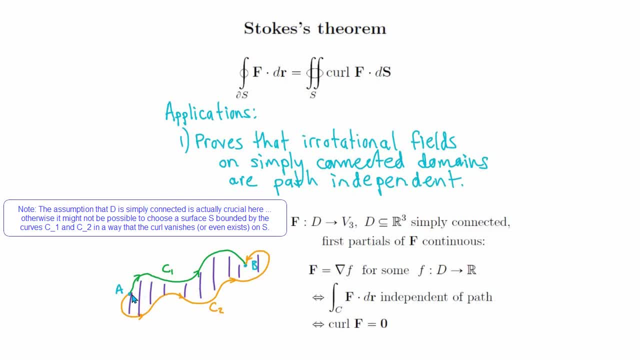 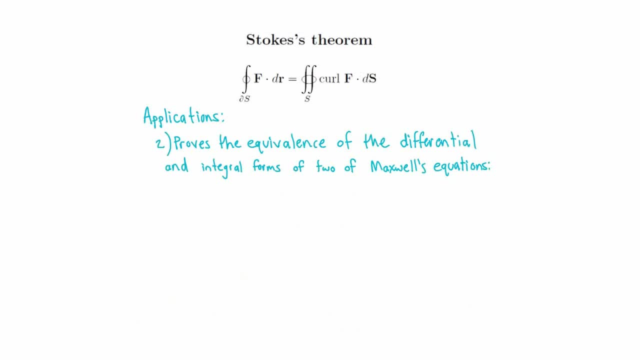 integral of f dot dr along C1 is equal to the line integral of f dot dr along C2.. In other words, line integrals of the vector field are independent of path. Another application which I think a lot of you will like is that Stokes' theorem proves the equivalence of the differential and integral forms. 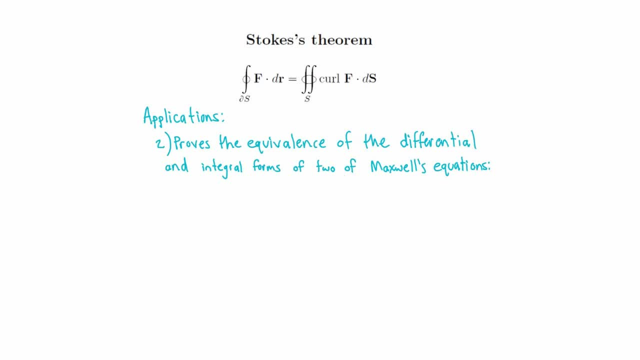 of two out of four and the integral of the vertical. This is a very simple and easy way out of four of Maxwell's equations. The other two out of the four equations, by the way, are going to be covered by the divergence theorem in the next video. The two equations that we want to